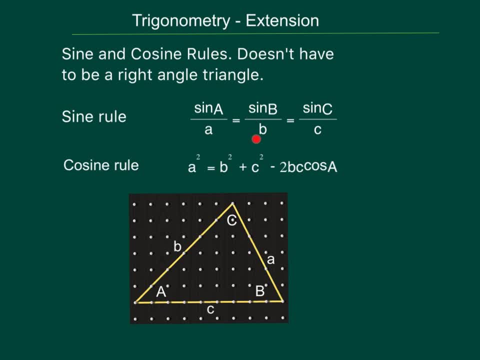 of those together. So I could use sine A over A equals sine B over B. Or I could use sine B over B equals sine C over C. Or I could use sine A over A, equals sine C over C. What do all those C's and A's and B's mean? Well, on a triangle like this one, down below the 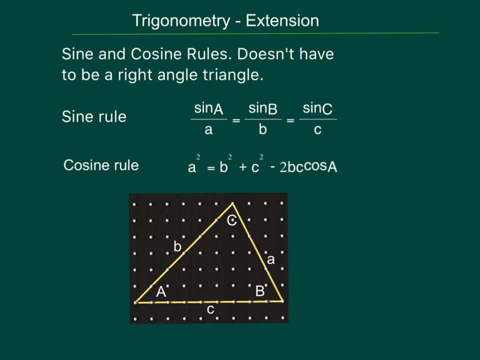 capital A, the capital B and the capital C are angles. The lowercase a, the lowercase b and the lowercase c are sides And you can put them wherever you like, so long as the lowercase c is opposite the capital C. the lowercase b is opposite the capital B. 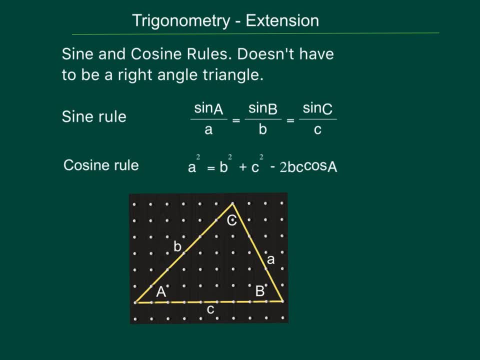 and the lowercase a is opposite the capital A. The second rule, the cosine rule, says that A squared equals B squared plus C. squared minus two, B, C cos A. This rule looks a little bit like Pythagoras's rule, Doesn't it? 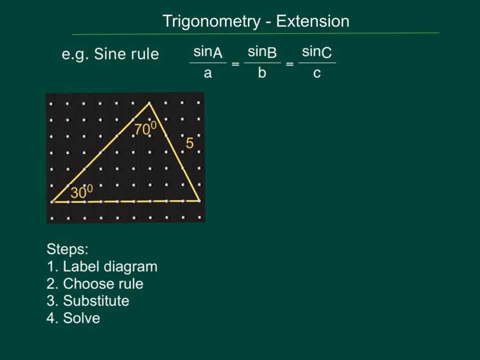 To use either the sine rule or the cosine rule, you must first of all label the diagram. So I'm going to start by labeling this side, this angle A, this side A, this side B and this angle B. I don't need to label C or C because I'm not going to use them, So I'm 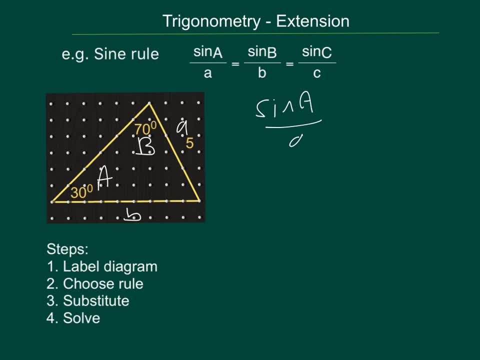 using sine A over A equals sine B over C, And I just need to substitute Sine 30 over 5 equals sine 70 over B. If I transpose the equation, I'll end up with B equals sine 70 over sine 30 over B, And I just need to. 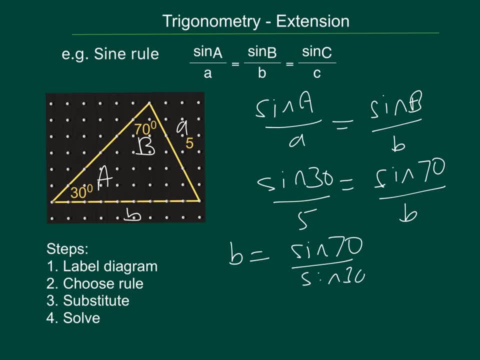 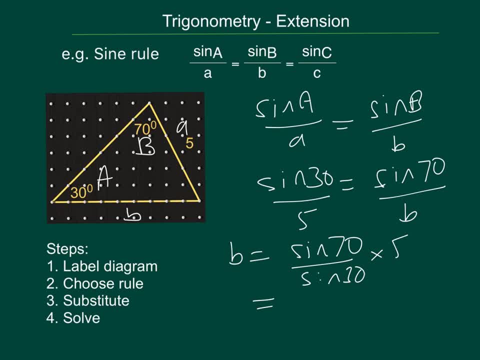 So I go to the generate line in the ів and I'm going to use the B bordered answer. O puedo lamentar? substituted 30 degrees, 70 degrees and 5 degrees and then solved the equation made B the subject. 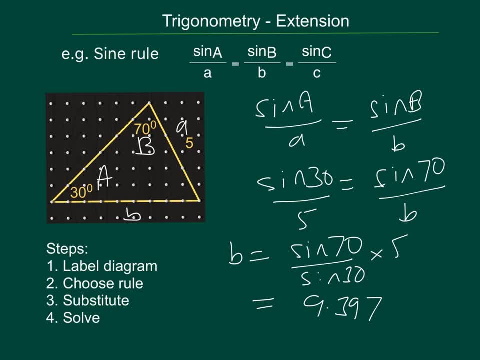 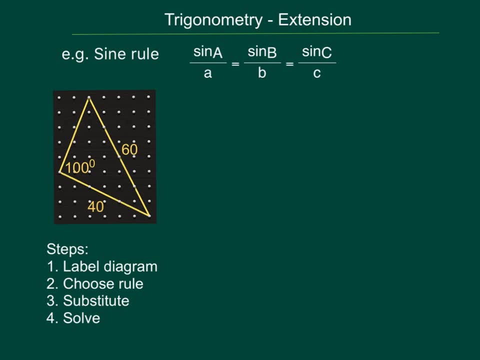 here it is and then calculated the answer. Here's another example. Maybe you could stop the video and see if you can work it out before I show you how to do it. So, assuming that you've done that, I'm going to follow the steps. Label a diagram. so I'll call this. 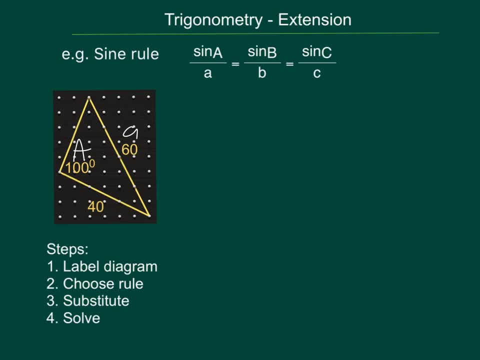 big A little a capital A, lowercase a, lowercase b capital B. And I'm going to try and find out what capital B is. So let's work, write down the equation: So sine A over A equals sine B over B, because I've got A's. 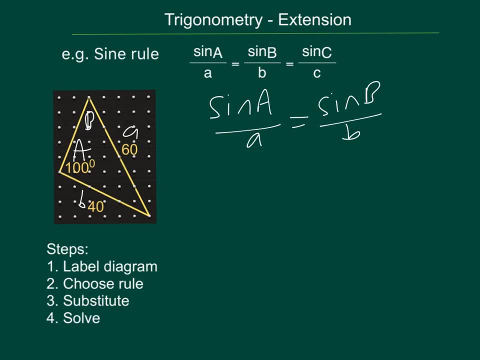 and B's and I need to then. well, I've chosen the rule, so now I need to substitute: So sine 100 over 60 equals sine B over 40. So I'll rearrange that to make sine B the subject, So sine. 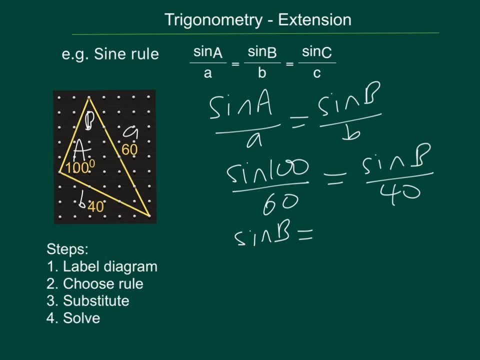 B equals 40 by sine 100 divided by 60, and the answer to that part is 0.6565.. Now that's what sine B is. So we need to get B. so I do inverse sine of both sides, Inverse sine of that side, inverse. 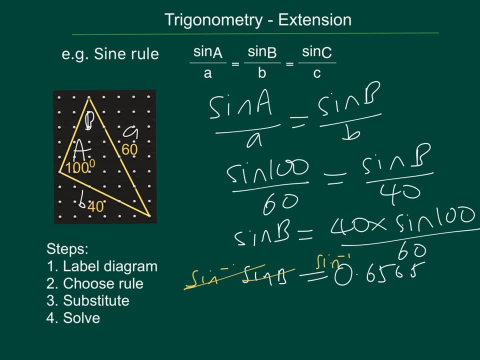 sine of that side. These two cancel, which is why we did it. So we end up with just B equals inverse sine of 0.6565, which is 41 degrees. Here's an example using the cosine rule. So again, I label a diagram So this can be. 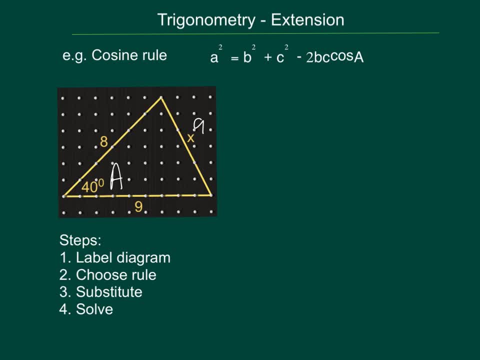 capital A, this can be lowercase A and this can be C and this can be B. So the rule is A equals B squared plus C squared minus 2BC cos A. So I'll substitute: A is X, so X squared. 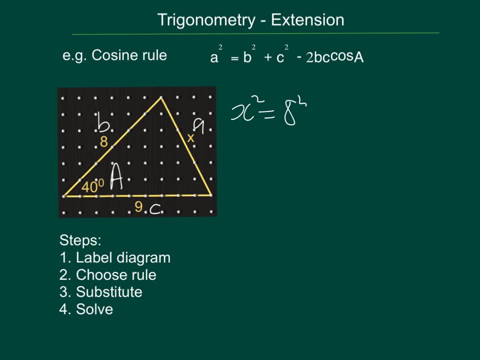 equals B squared, which is 8 squared, plus C squared, which is 9 squared minus 2 times BC, which is 2 times 8 times 9, multiplied by cosine of 40 degrees. So, working that out, 8 squared is 64,. 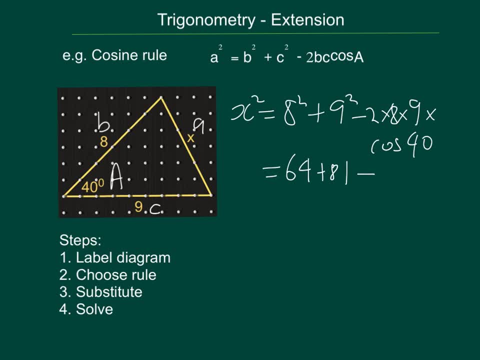 9 squared is 81.. This bit on the end is equal to 110.31.. So altogether that makes 34.69.. So that means we've got X squared equals 34.69.. Now we need to find X, so we have to. 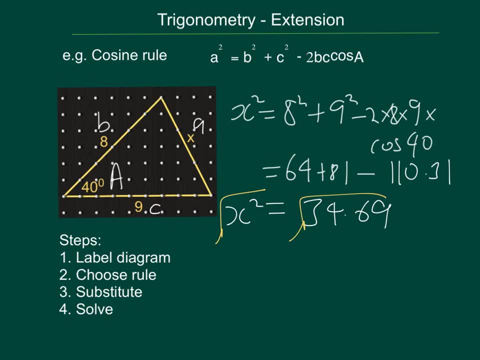 square root. both sides, On the left, the square and the square root are inverses, so I just end up with X, And on the right the answer will be 5.89.. So this example is a little bit different. So I'll label my diagram. There's an A here. 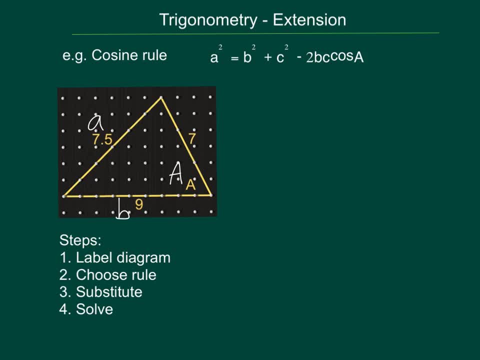 a lowercase A here. this one can be B and this one can be C. So if I substitute in, I'm going to get 7.5 squared for A, squared 9, squared for B, squared plus, 7 squared for C, squared minus. 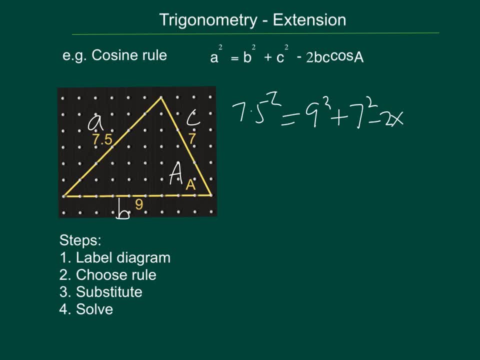 2 times A times B, which is 63, cos A. Now, because A is the unknown, I need to rearrange the equation to make a cos A the subject. But before we do that, we'll do a bit of tidying up. 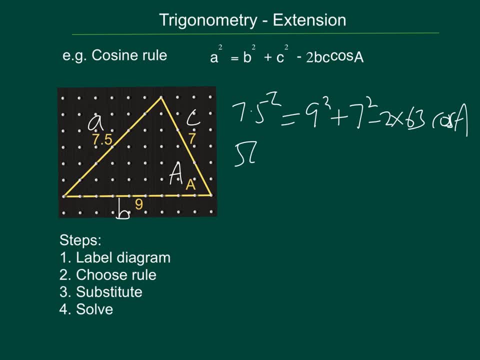 So 7.5 squared is 56.25.. And 9 squared and 7 squared is 130 minus 126 cos A. Therefore, cos A is going to be equal to 56.25 minus 130 divided by minus 126,.